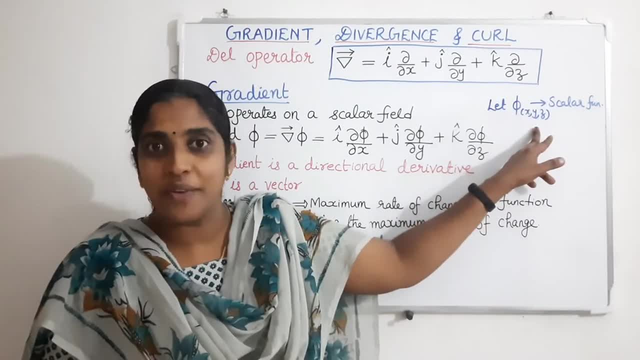 that b, phi, x, y, z, for example, potential function. that is a scalar function. So this del is operating on this scalar function, phi. but we can consider this del operating on the scalar function phi. So we can consider that b, phi, x, y, z, for example, potential. 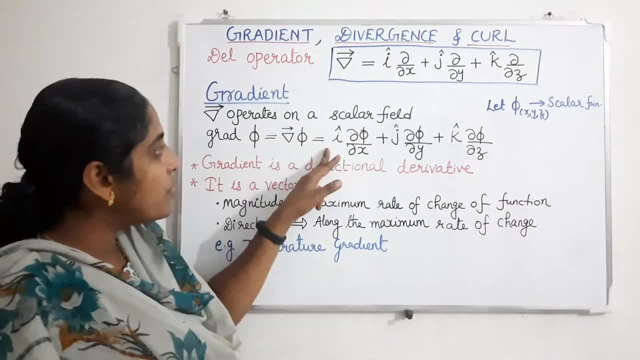 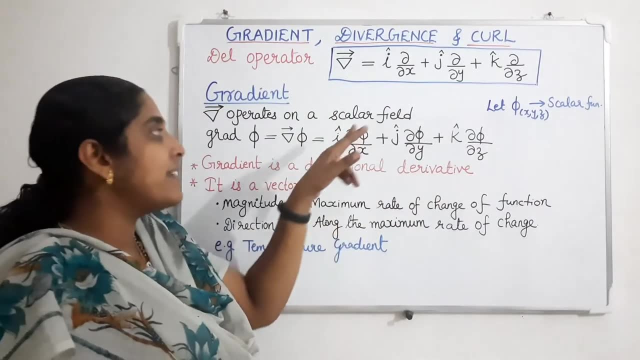 phi leads to the gradient. So that is equal to i dou by dou x plus j dou by dou y plus k dou by dou z that is operating on phi. that is i dou phi by dou x plus j dou phi by dou y plus k dou phi. 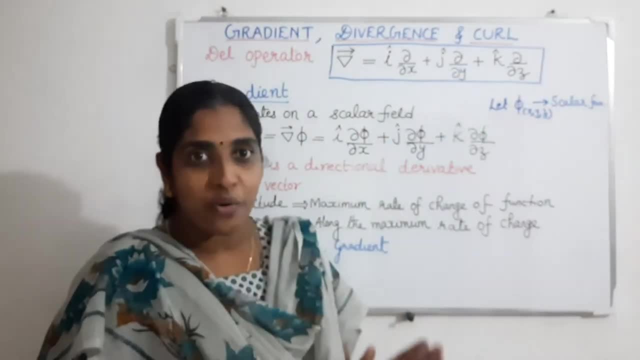 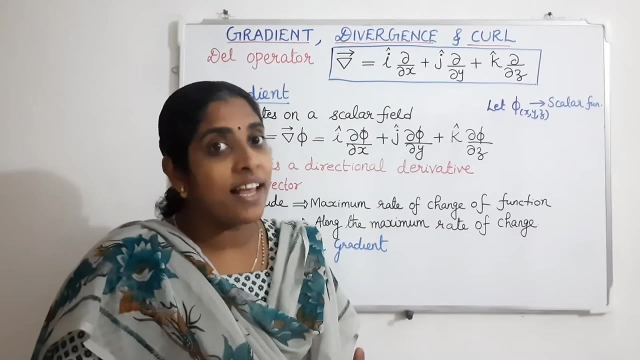 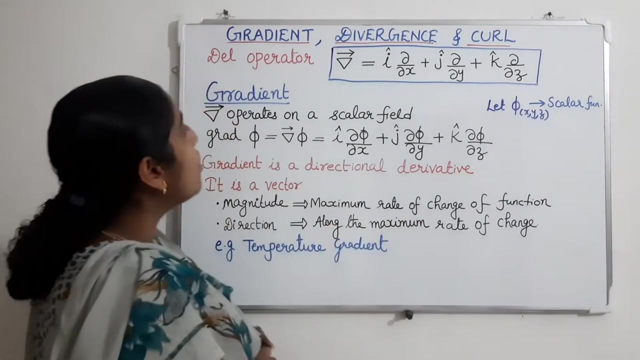 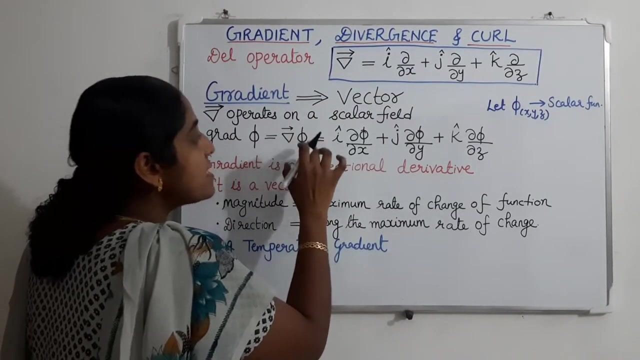 by dou z, where this phi is a scalar quantity. When this del is operating on this scalar quantity, whatever we are getting is a scalar or a vector. it is a vector quantity. See this? they have a direction i, j, k. So the answer is a vector quantity. So when del operates on this, 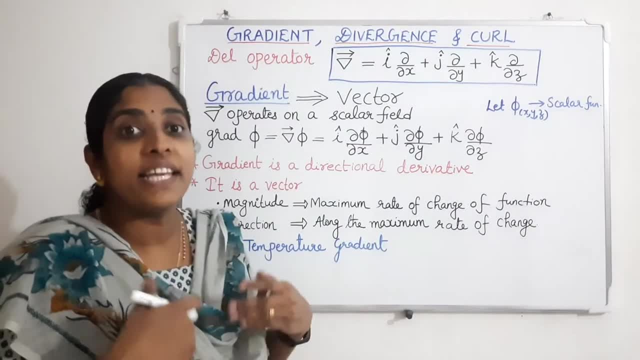 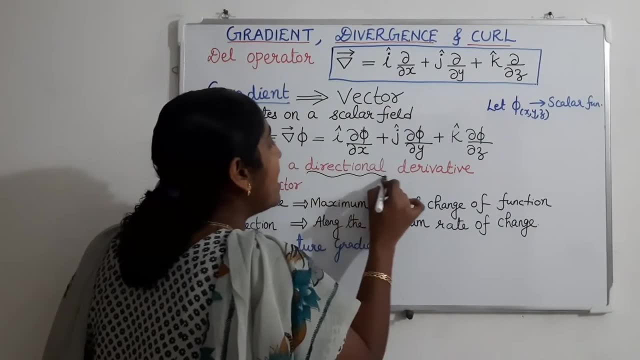 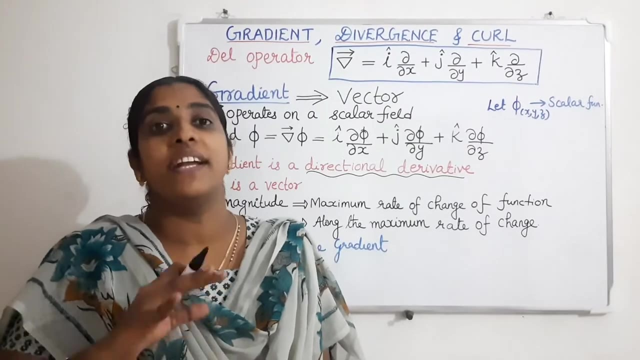 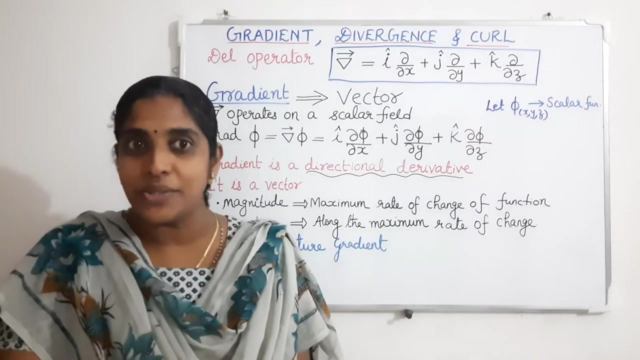 scalar function, phi, it gives some direction to that quantity. So we can call this gradient as a directional derivative. So gradient is a directional derivative. it is a vector quantity. When del operates on a We are getting a vector. If it is a vector, we have a magnitude and a direction. then what will? 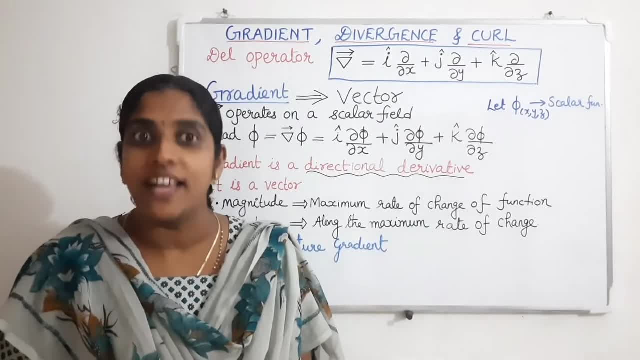 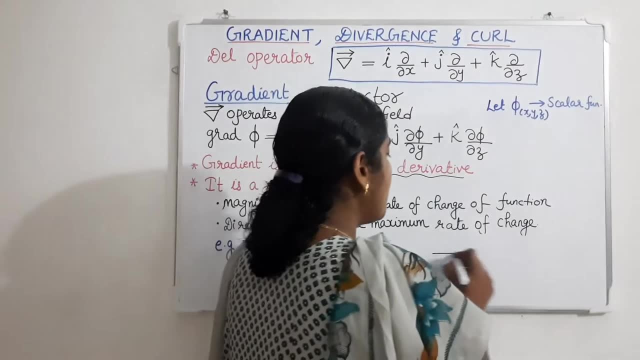 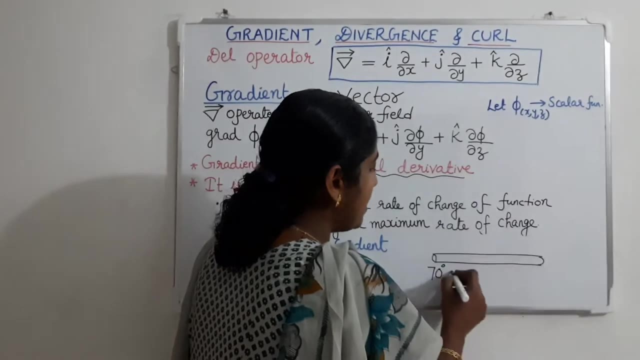 be the magnitude and the direction of that gradient. What is the physical significance of this gradient? For example, we can consider a hot iron piece. Let the ends of this hot iron rod are at a different temperature. Let at one end the temperature is 70 degree Celsius. 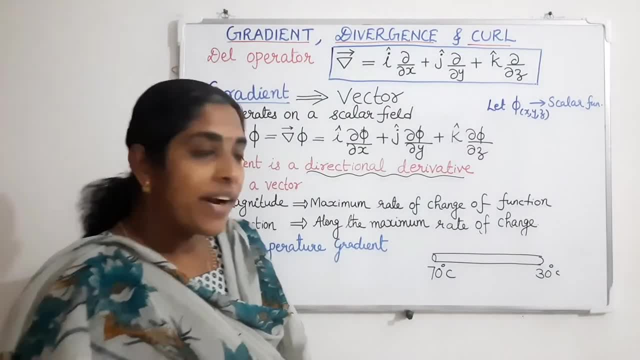 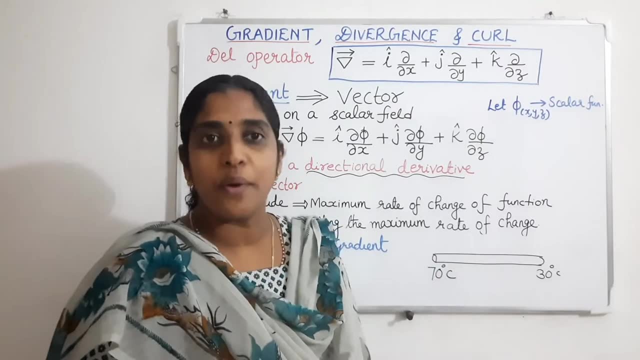 and at the other end let it be 30 degree Celsius. Then what happens? The heat energy will flow from the higher temperature region to the lower temperature region until the temperature on the rod becomes uniform, that is, it becomes 50 degree Celsius, Then the 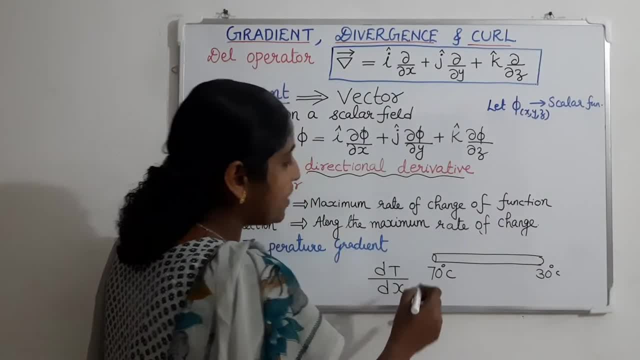 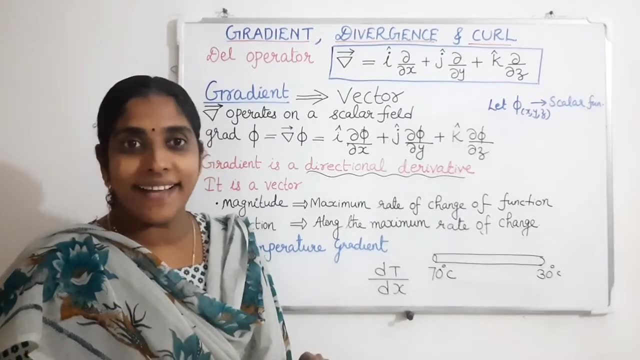 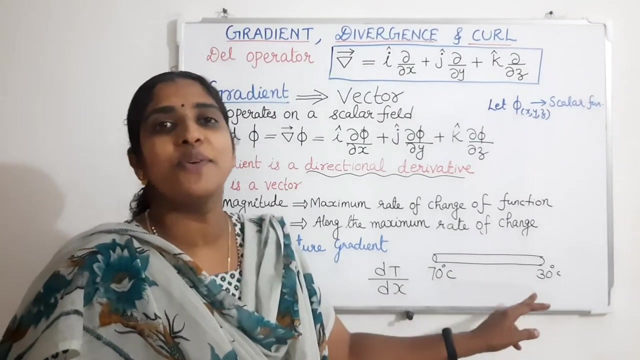 change in temperature per unit length of this rod is known as the temperature gradient. This temperature gradient will have a magnitude and a direction. Then what will be the magnitude and what will be the direction? Magnitude will be the maximum rate of change of this. 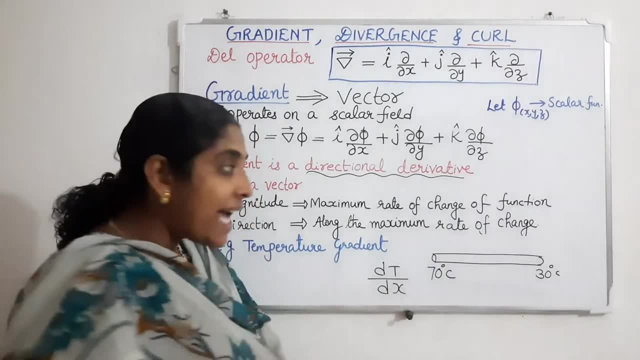 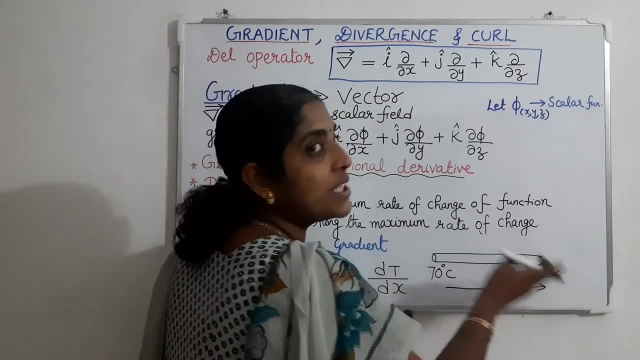 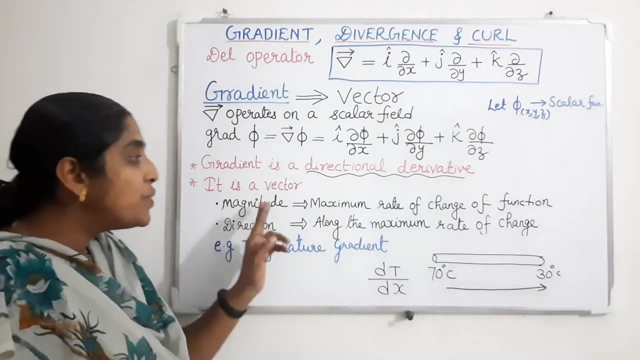 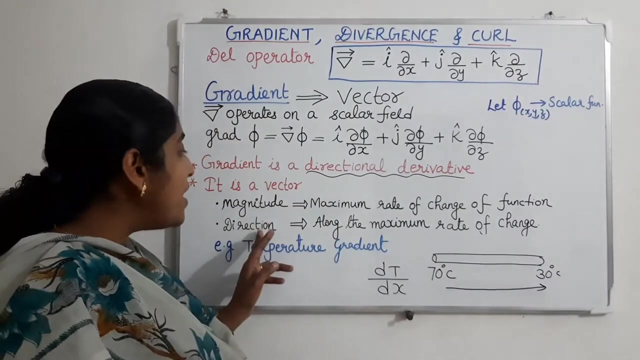 temperature and direction will be the direction along which that change occurs, that is, along the direction from 70 degree to 30 degree. So in this gradient it is having a magnitude and direction. So the magnitude will be the maximum rate of change of that scalar function and direction will. 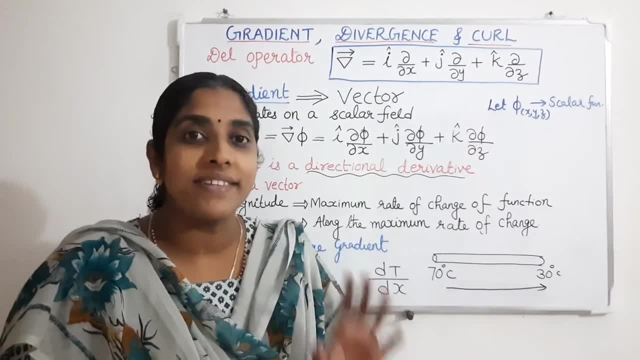 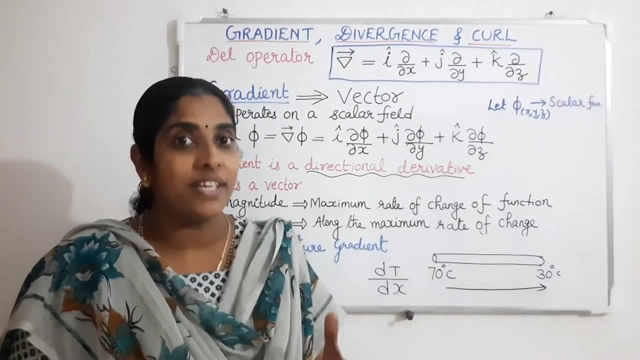 give along which direction that maximum rate change occurs. So in this gradient it is having a magnitude and direction. So we can call gradient as a directional derivative. It is a vector quantity. It is having a magnitude and direction. The magnitude gives the maximum rate. 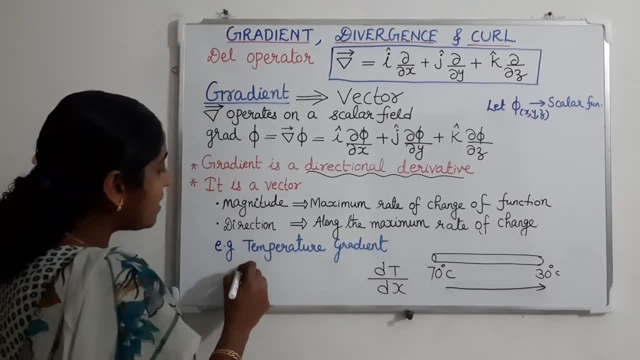 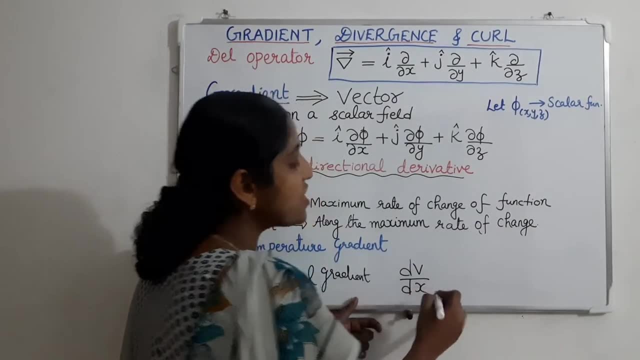 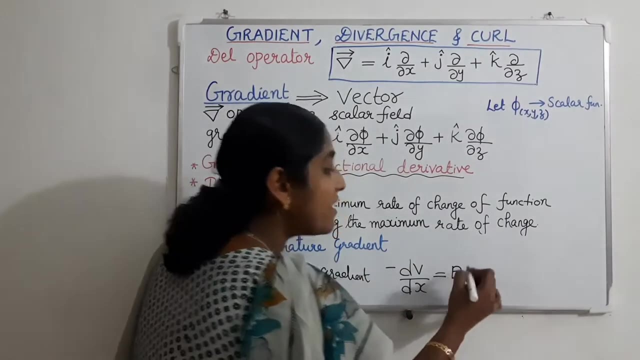 of change of that function. We can also consider another example: potential gradient. What is potential gradient? Potential gradient is a change in potential per unit length. I mean electrostatics. you have seen that the negative of this potential gradient is the electric field. This is in one dimension. If we are considering in three dimension- electric field. 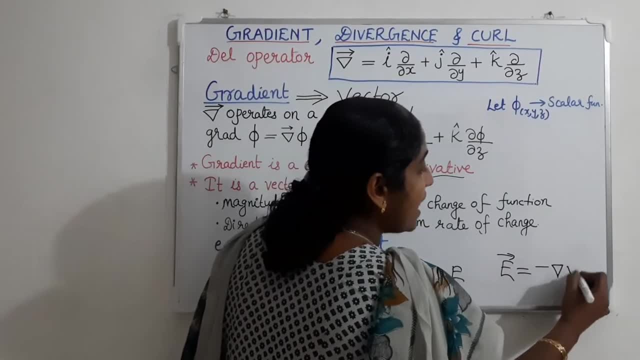 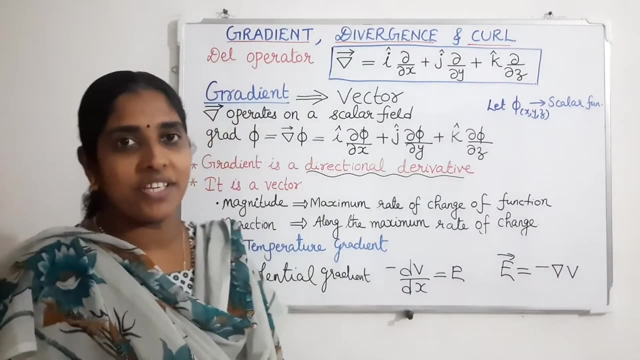 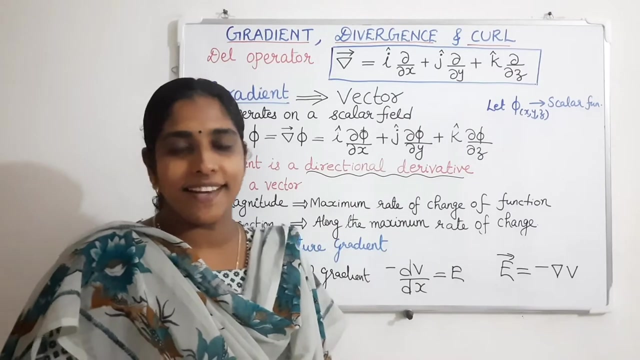 vector. we can write as negative of the gradient of the scalar function v, So it is a vector quantity. that is, gradient of a scalar function is a vector quantity. The magnitude has the maximum rate of change of that function and direction has the direction along which that change occurs. 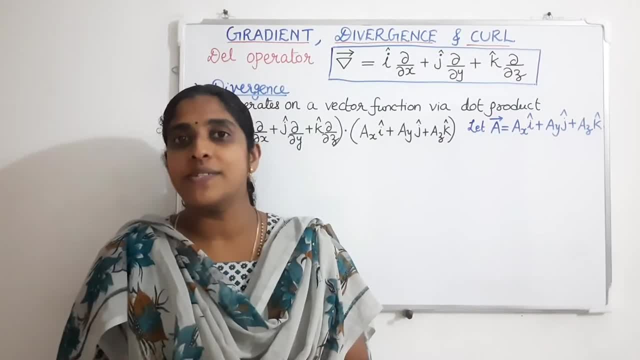 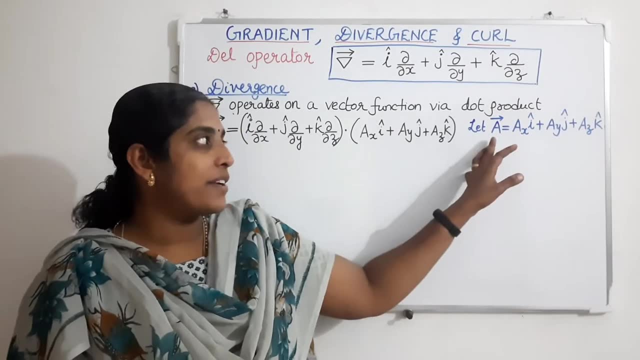 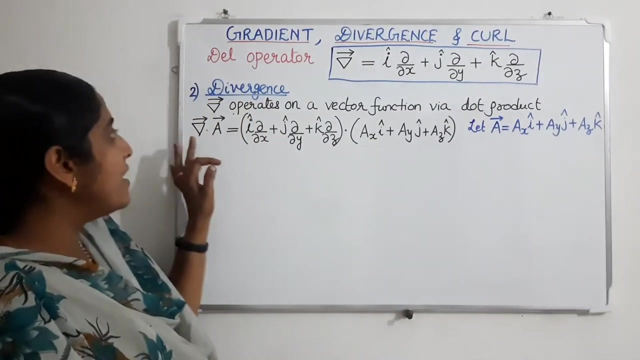 The second one is divergence. When del operates on a vector function by dot product, the resultant is known as the divergence. So we can consider a vector function a vector that is equal to a, x, i plus a, y, j plus a, z, k. So here del is operating on this. 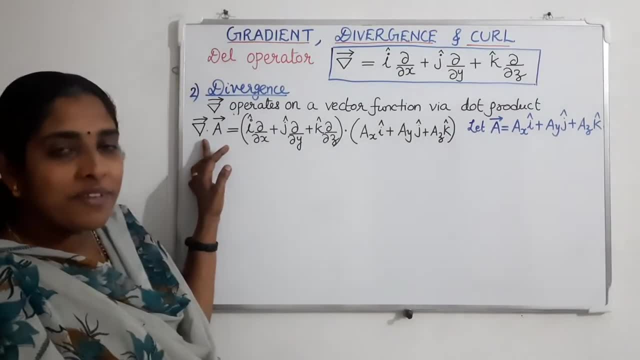 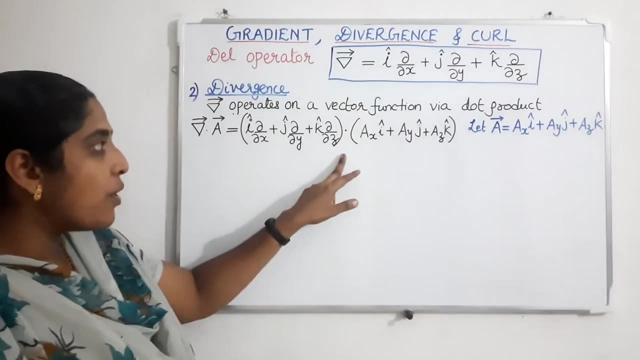 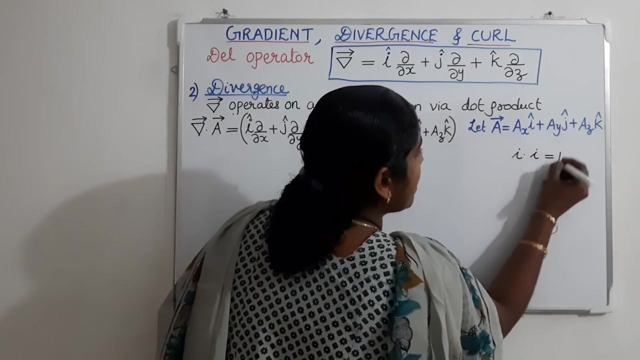 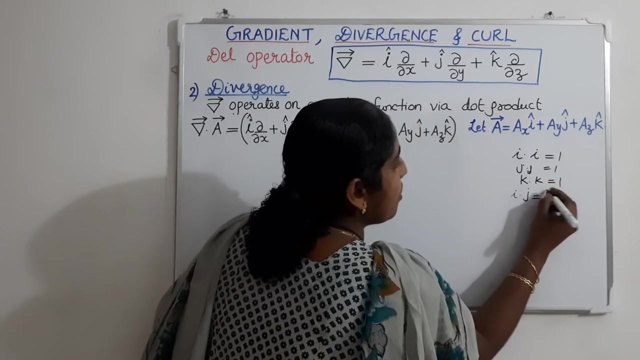 vector function a by dot product, then what we will get: i dou by dou x plus j dou by dou y plus k dou by dou z, that is del dot that vector a x, i plus a y j plus a z k. We know that i dot i is equal to 1, j dot j is equal to 1, k, dot k is equal to 1 and i dot j, j dot k, k, dot i is equal. 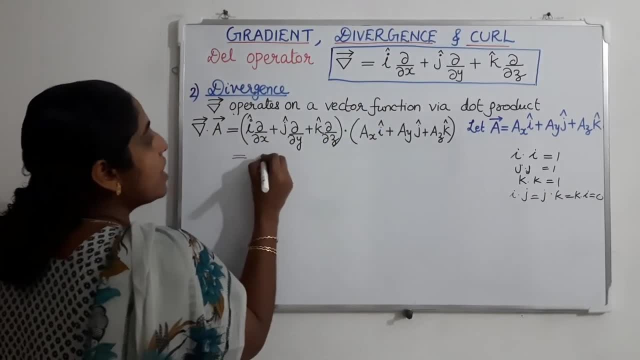 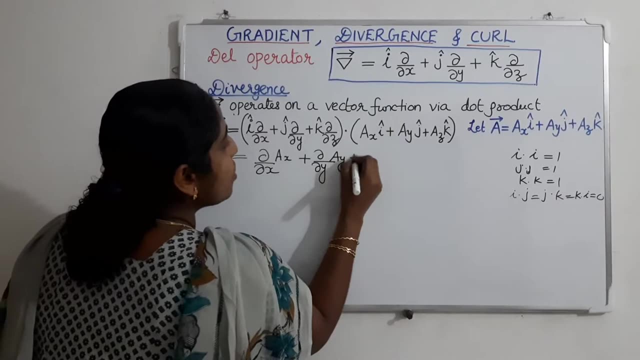 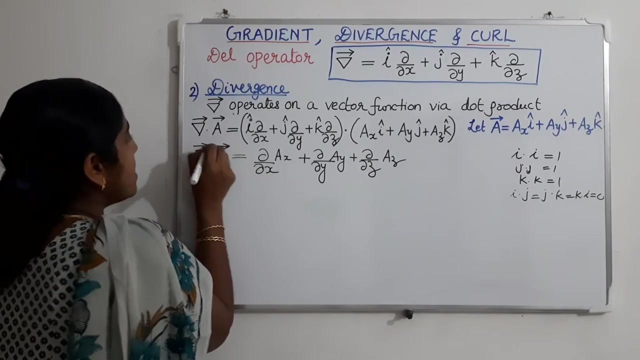 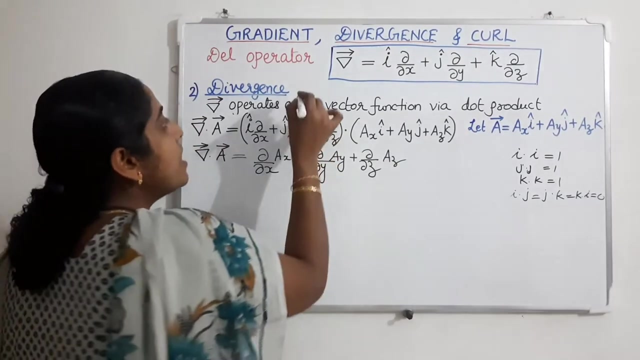 to 0. So, on taking the dot product, we will get dou by dou x of a x plus dou by dou y of a, y plus dou by dou z of a z. So del dot a, that is, divergence, is a scalar quantity. In this resultant we are not getting the direction. So we can say that the 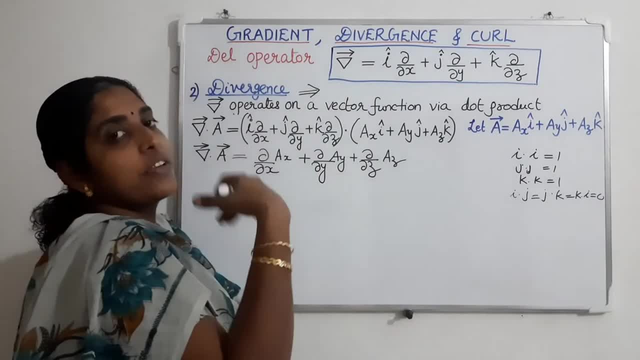 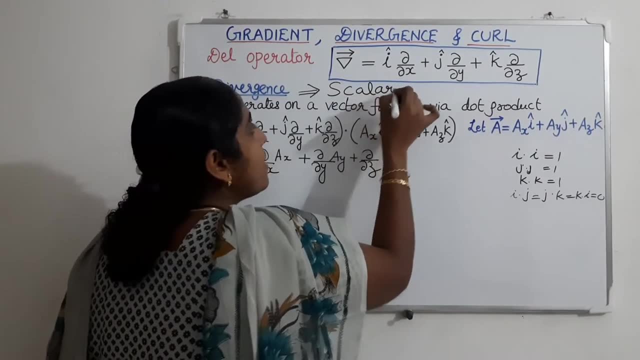 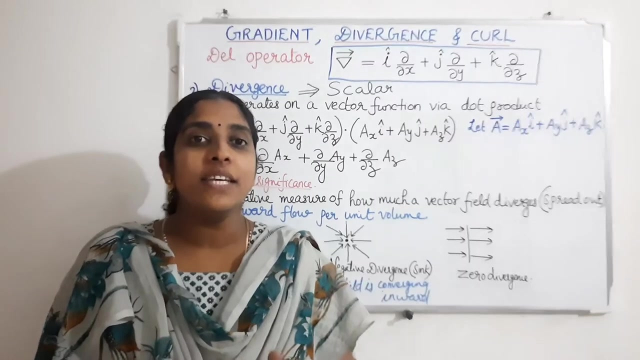 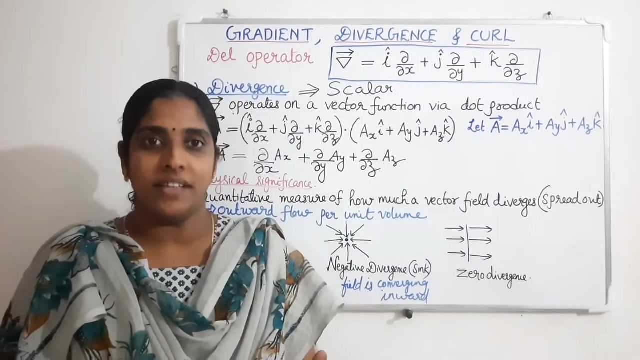 resultant of del operation on vector function by dot product is a scalar, Then what will be the physical significance of this divergence? The physical significance of divergence is that it gives a quantitative measure of how much a given quantity is diverging at a given point, That is, how much that a quantity is spread out For. 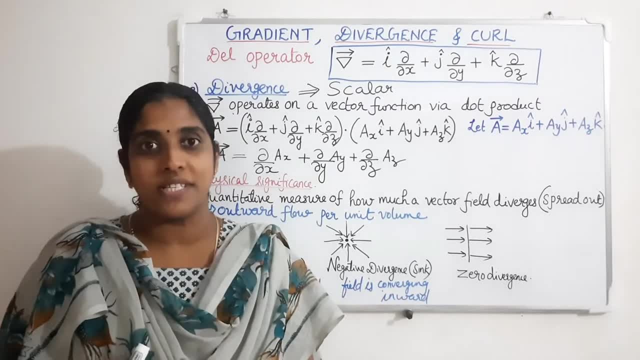 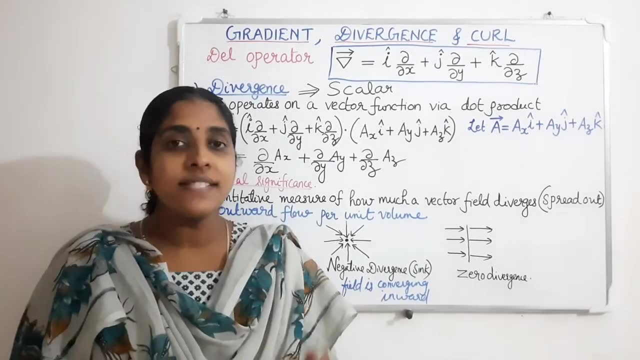 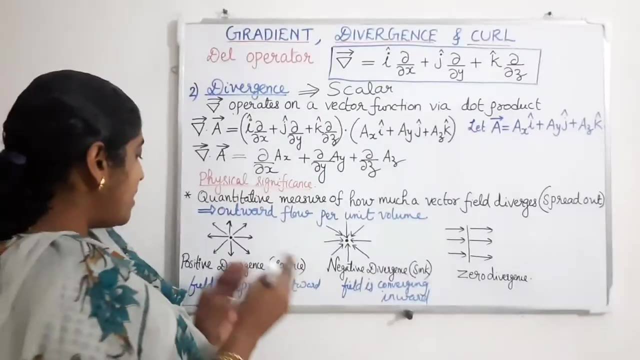 example, if you are considering the divergence of fluid velocity, that will be the quantity of the fluid flowing out at a given point, We can say the divergence as a positive when this flow occurs outward, That is, if the field is spreaded outwards, that divergence is positive. 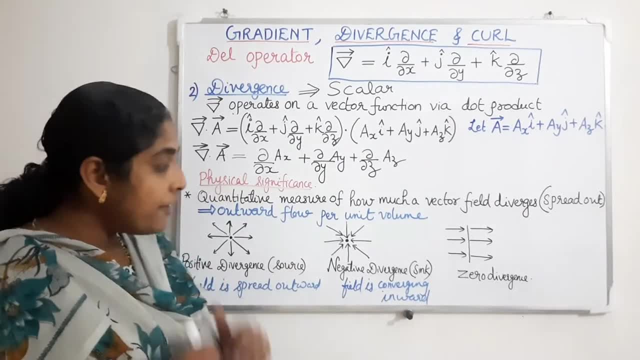 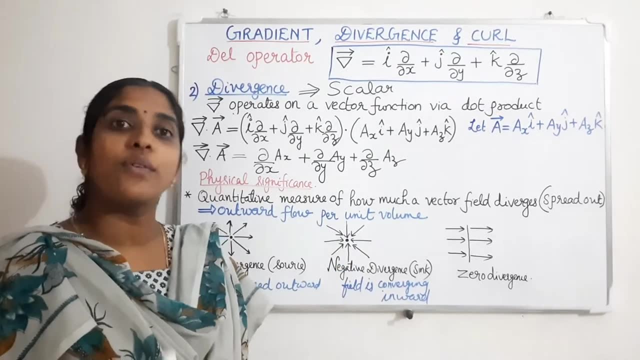 It is a своим divergence, or we can call it as source. If the field is converging inward, that divergence is known as negative divergence or sink. There is one more divergence: zero divergence, that is, if the field entering is equal to the field leaving, then it is zero. 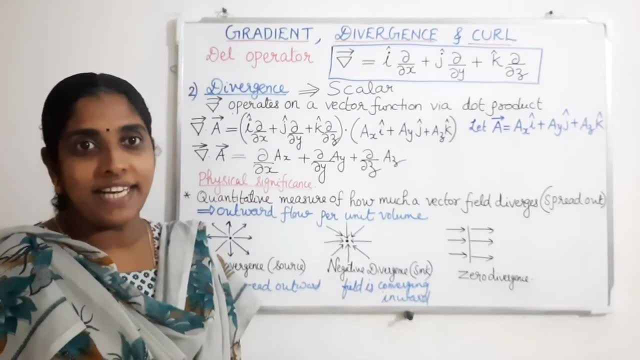 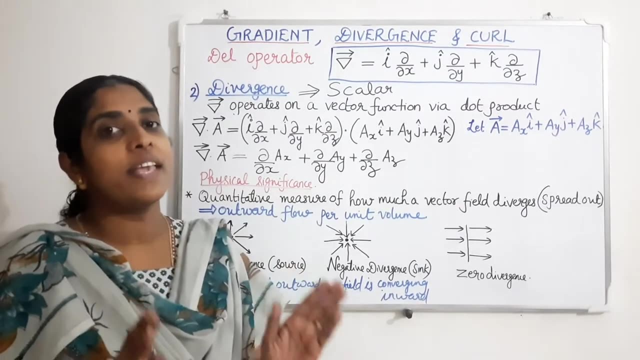 divergence. So the physical significance is that it gives how much a vector quantity is diverging, That is, it is a outward flow inside the vector from the, the, our emidium. So will bebokki into a good일 rounded flow minus point k, z, with reference to z, a, d, e, r, d, x, d o. So the difference is, that is the overall Denver divergence. psi d, d, e, d a, always Nichou-M Solar. this mean it will regard� z. So then a bit will be those all as looks like this, So as, for example, if the motion of the problem 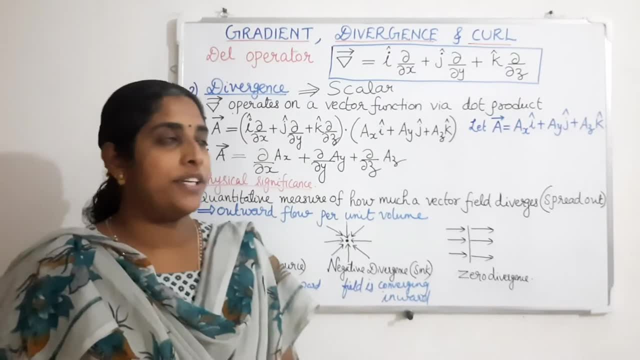 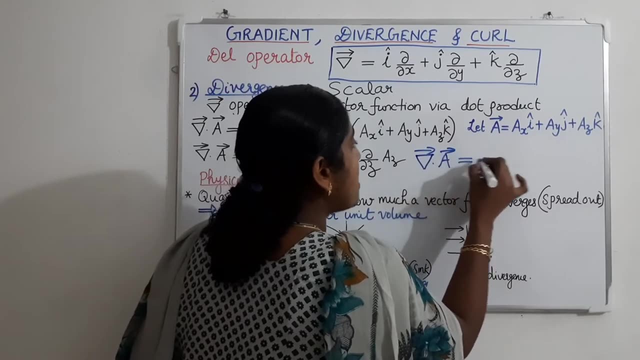 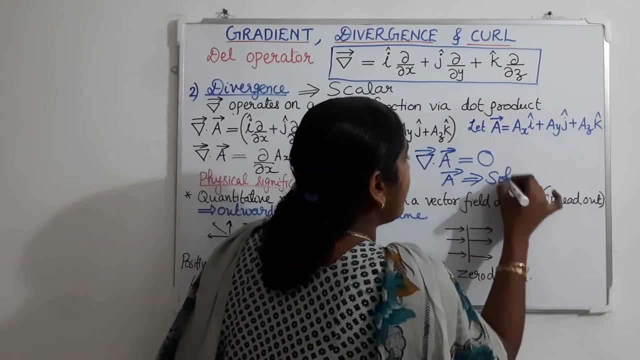 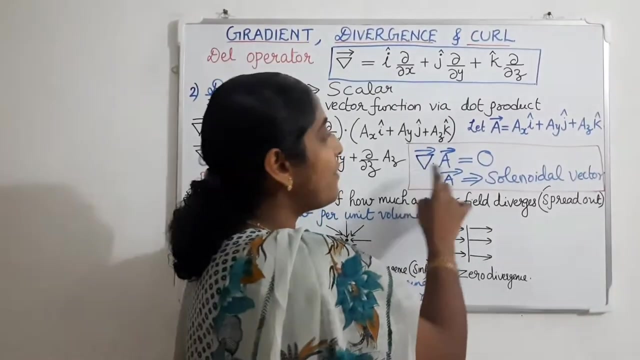 flow per unit volume. Another important point is that if we are taking the divergence of a vector quantity and if we are getting the answer as 0,, then this A vector is known as solenoidal vector. So for a vector to be solenoidal, the condition is that the divergence of that vector quantity 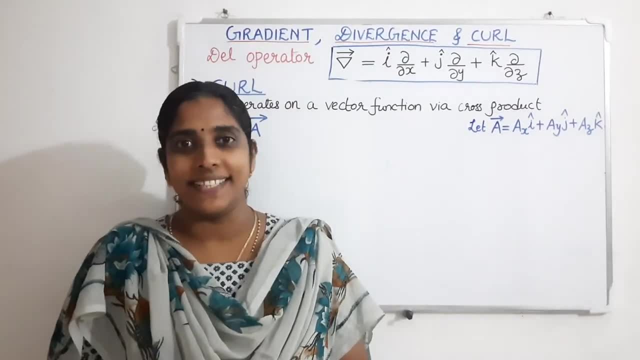 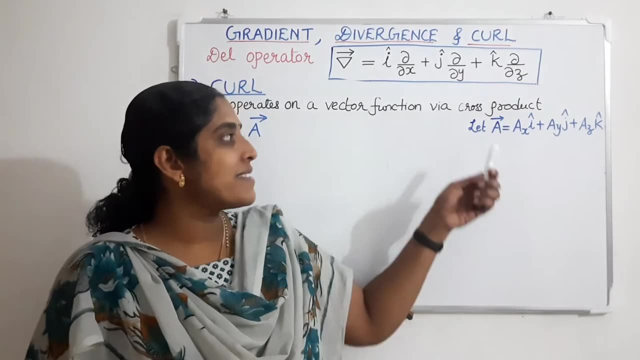 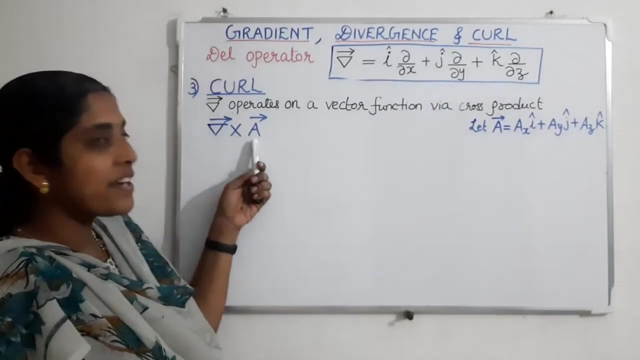 must be 0.. The third one is curl. When del operates on a vector function via cross product, the resultant is known as the curl. So we can consider the same vector function A vector that is AXI plus AYJ plus AZK. This del operates on this vector function by cross product. Then what? 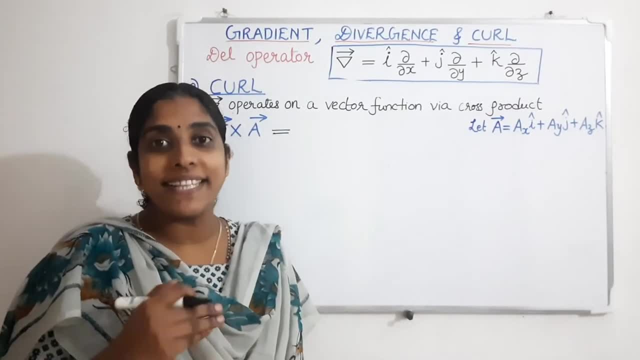 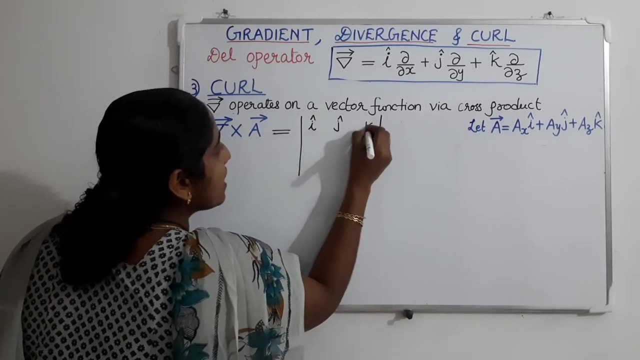 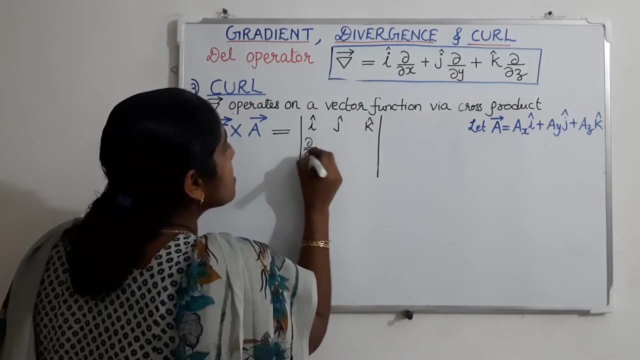 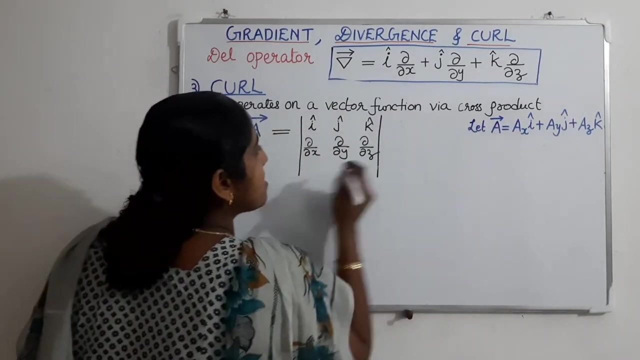 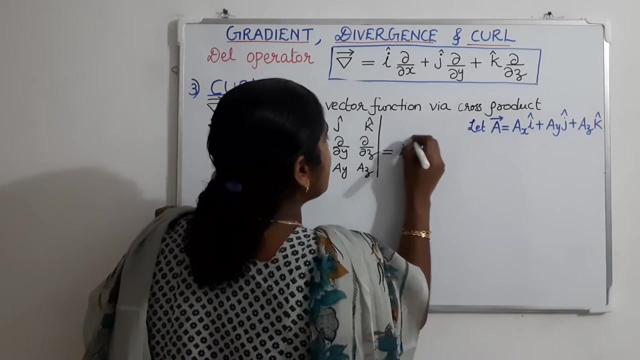 will be the resultant, The cross product we can find by the determinant method, that is determinant of IJ. The components of del along IJK are dou by dou X, dou by dou Y, dou by dou Z. The components of vector A along IJK directions are AX, AY, AZ. So the answer will be: I into dou by dou Y of AZ. 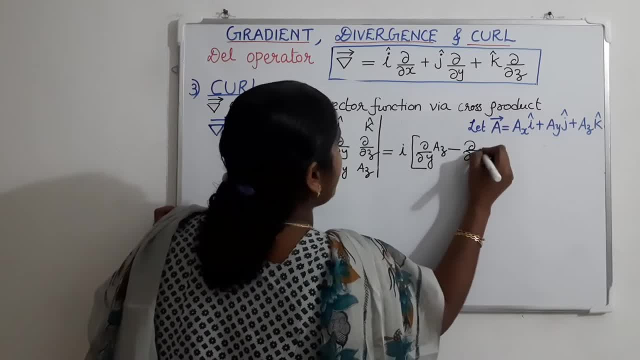 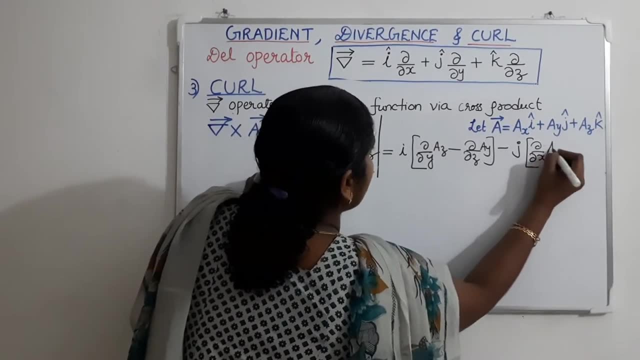 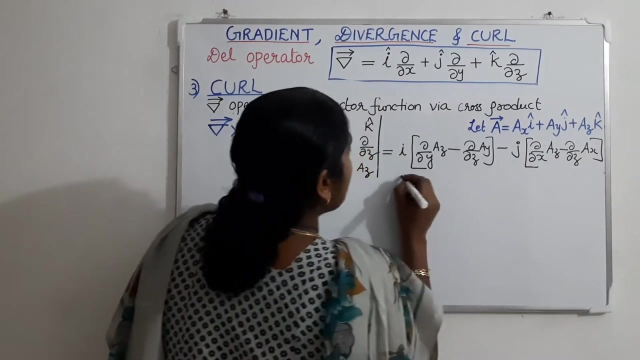 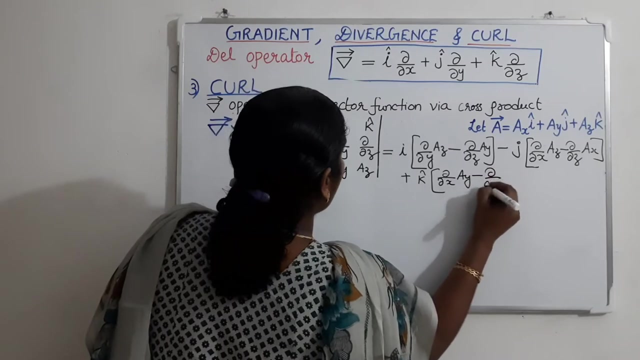 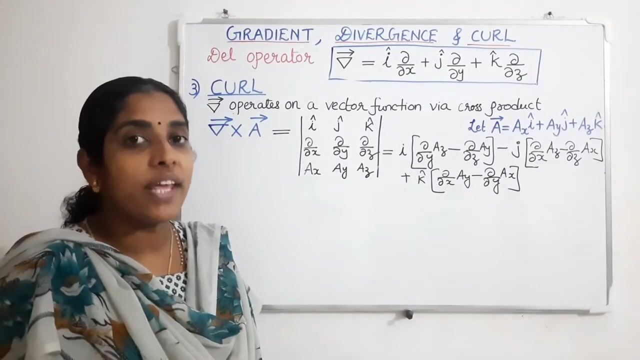 minus dou by dou Z of AY, Minus J into dou by dou X of AZ, minus dou by dou Z of AX, plus K into dou by dou X of AY, minus dou by dou Y of AX. So the resultant is a vector or a scalar. It is a vector quantity. 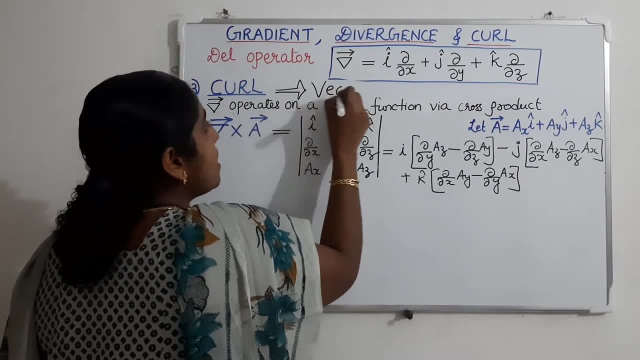 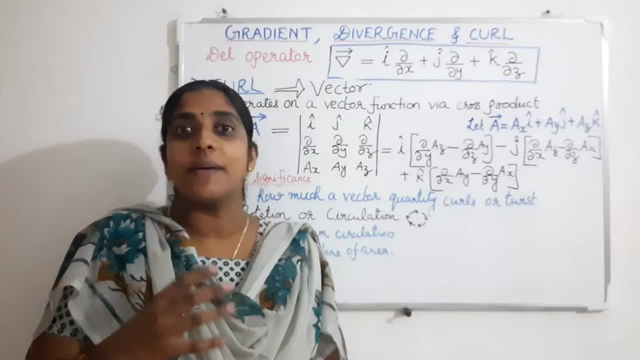 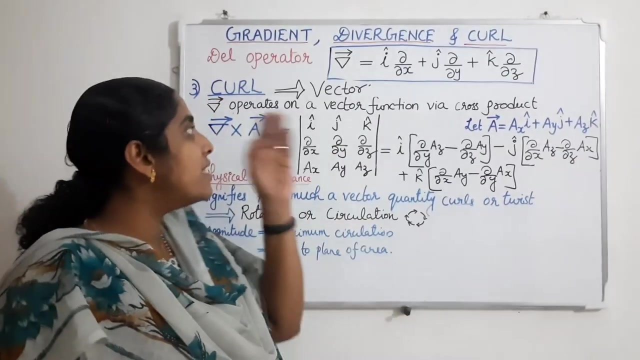 That is, curl is a vector quantity, Then what will be the significance of this curl? The word curl is related with something that is twisting or it is going a spiral, For example we are telling curly hair. So the physical significance of curl operation here is that it gives how much a vector 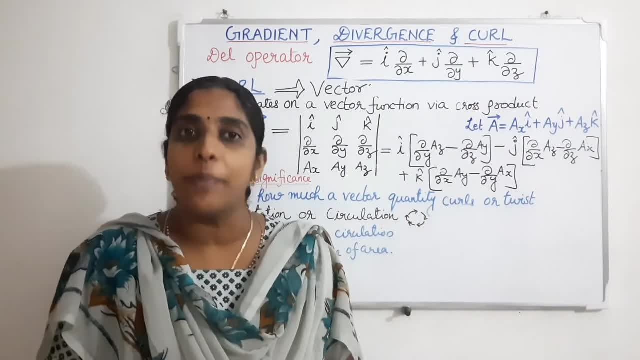 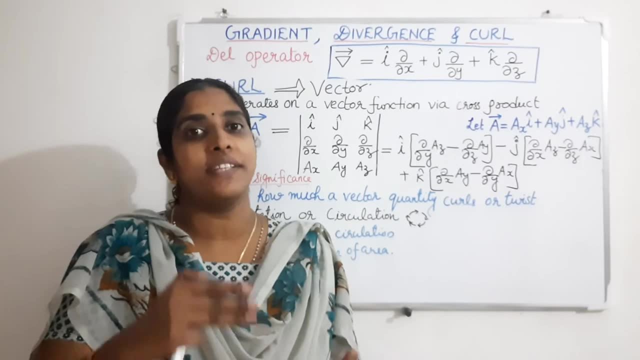 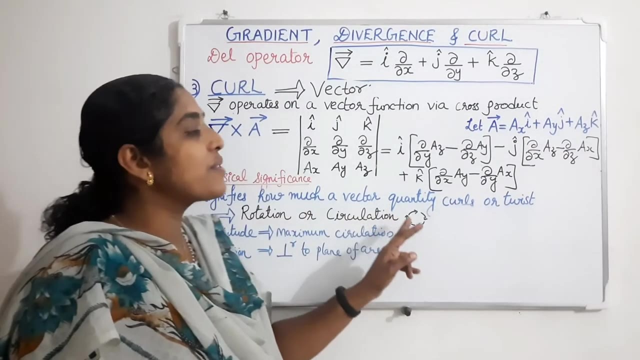 quantity curls or twists around a pointer. So when we are finding curl at a pointer that will give the circulation of that vector around that point or rotation of that vector around that point. So curl gives the rotation or circulation around a point. We have seen that. 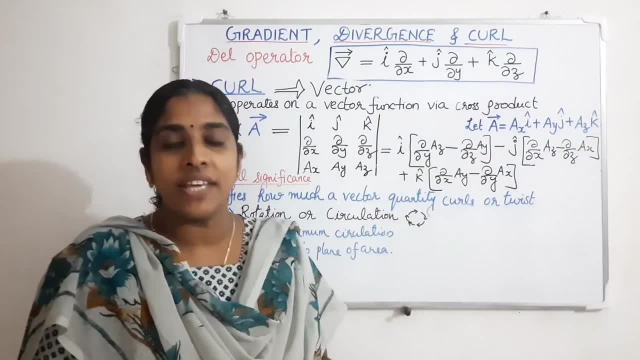 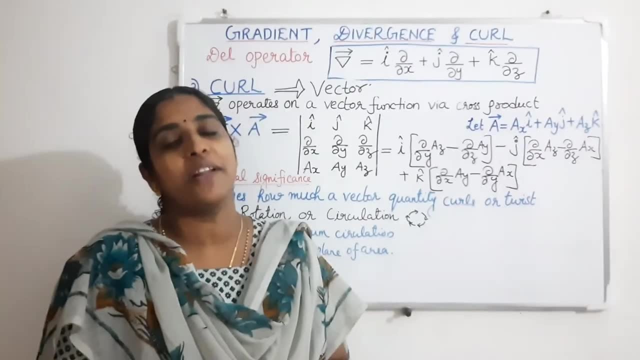 curl is a vector quantity, So curl is having a direction and magnitude. The magnitude will be the amount of maximum circulation around that point. And then what will be the direction of that curl? That will be perpendicular to the planar, So that is the direction of that.